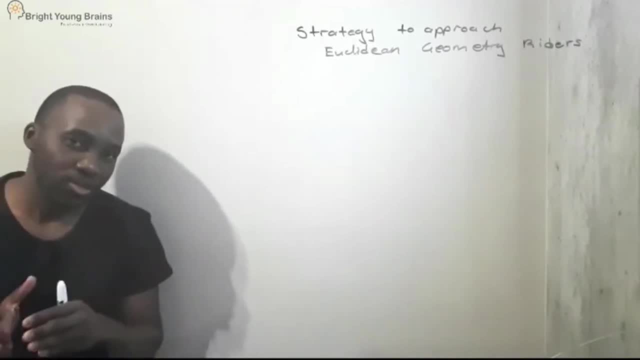 here. it is quite famous and it also has its own acronym. It's called Dr Keptown. So Dr Keptown is an acronym for Dr Keptown. Dr Keptown is an acronym for Dr Keptown. 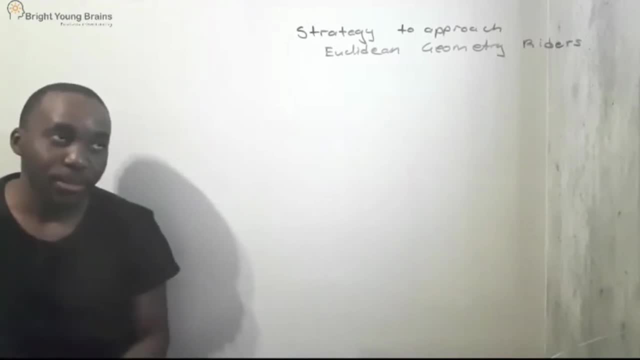 Dr Keptown is an acronym for Dr Keptown. I think you may have heard of it or something like that, but with Dr Keptown this is the acronym you want to remember: D-R-C-P-T. Dr Keptown, Keptown. 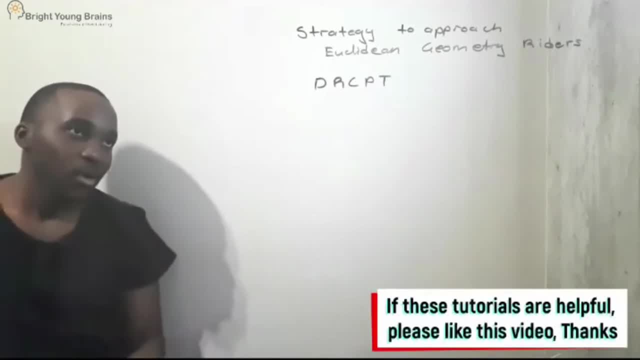 So anyways, with Dr Keptown, the one thing is, each of these letters represent one specific thing about circles and Euclidean geometry. So firstly, with D, D refers to diameter. so whenever you have Euclidean geometry equation, whatever your sketch looks like you want. 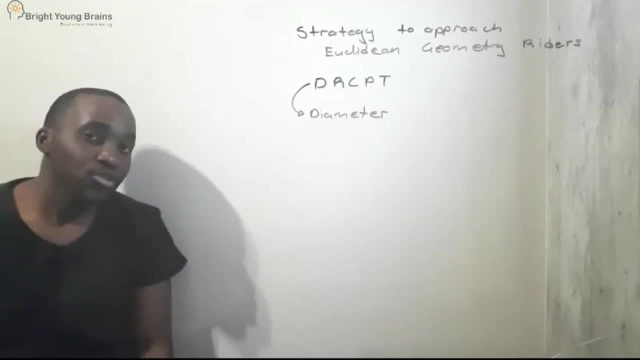 to look out for a diameter first. The reason is, the moment you look out for a diameter, you will be able to remember this theorem. This theorem says that a diameter of a circle subtends an angle of 90 degrees, or rather, an angle subtended by the diameter of a circle. 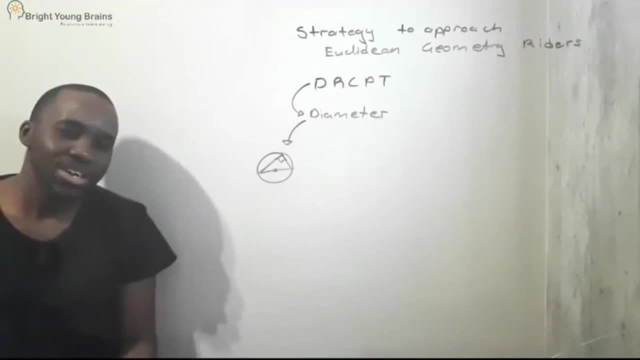 is equal to 90 degrees. So this is theorem 3.. There we go. The R stands for radius, in the sense that whatever Euclidean geometry sketch that you'll be given, you need to look for a diameter first. think of this theorem. 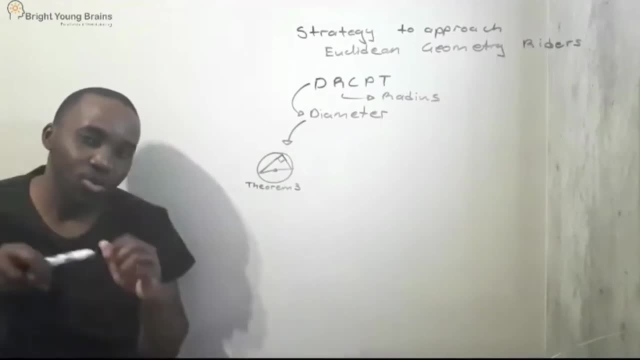 and then next, you need to look out for your radius, or irradiuses, or whatever you want to call them. So when you think of irradiuses, the one thing that should come to mind theorem 2.. Because theorem 2 states that an angle of 90 degrees is equal to 90 degrees, and 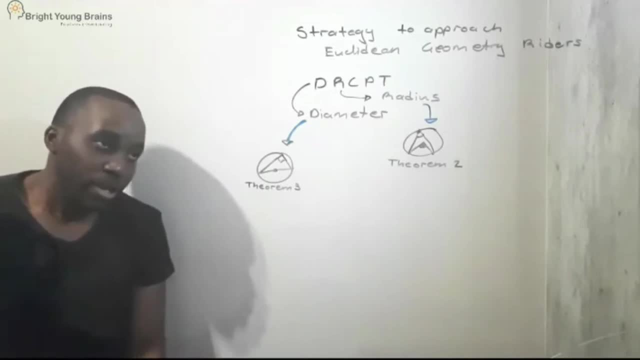 an angle at the center of the circle will always be double an angle at the circumference. Now the issue is this angle that will be at the center of your circle. We know that these two lines here will always be the radius of your circle. And apart from just remembering 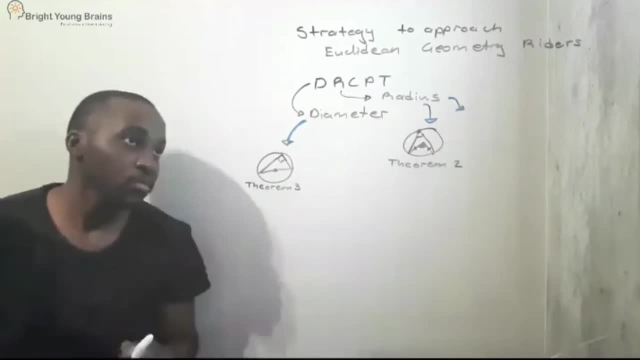 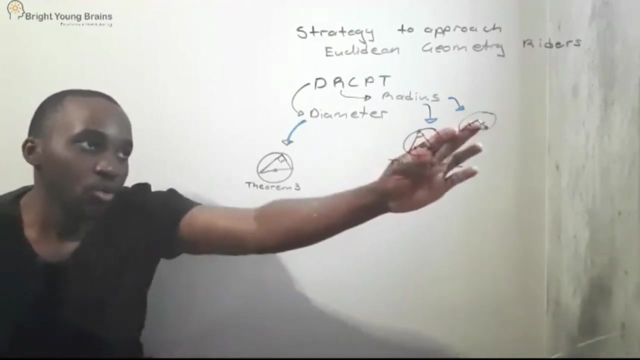 this law. we know that whenever we have a radius, we need to look out for an isosceles triangle somewhere in our sketch Because, remember, with an isosceles triangle you have base angles that will be equal to each other, because your lines there from the center. 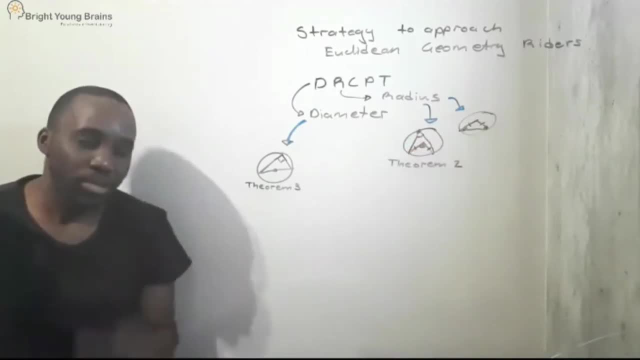 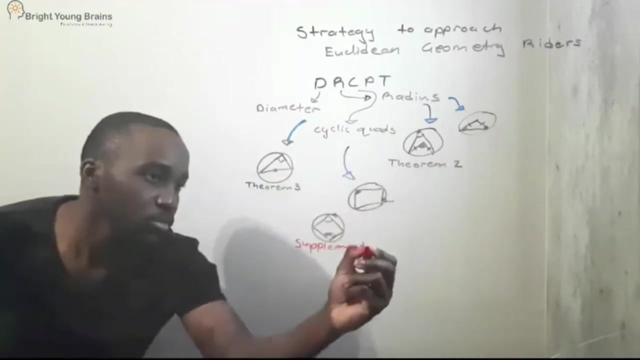 of your circle will be equal because they are a radii. They are both at the radius of your circle. So that's what R stands for, radius, C stands for cyclic quads. Now, with cyclic quads, we know that opposite angles will be supplementary, and we also know that. 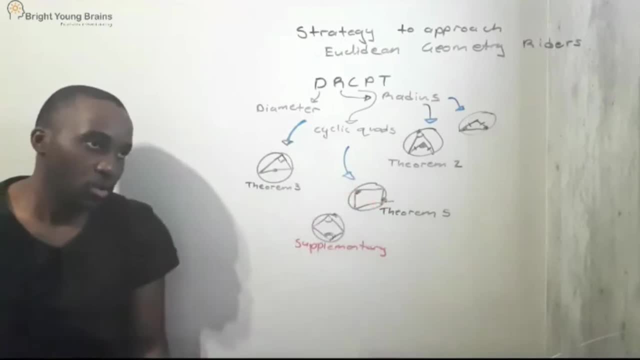 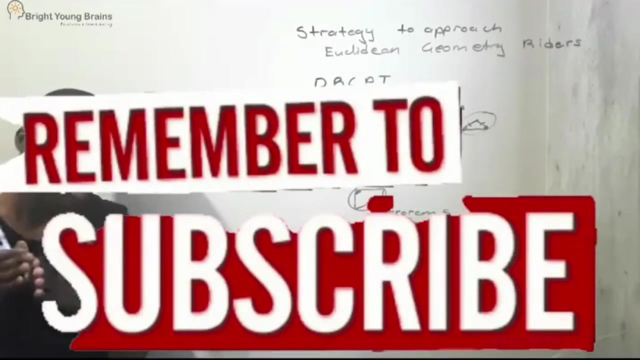 an exterior angle, a cyclic quadrilateral is equal to the opposite interior angle there. So when you think of D diameter, R radius, C, cyclic quads, your brain is already like working in terms of trying to feed information to you so that you'll be able to answer your Euclidean Geometric Question. 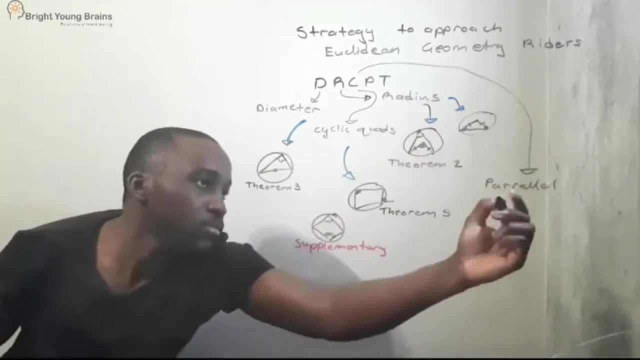 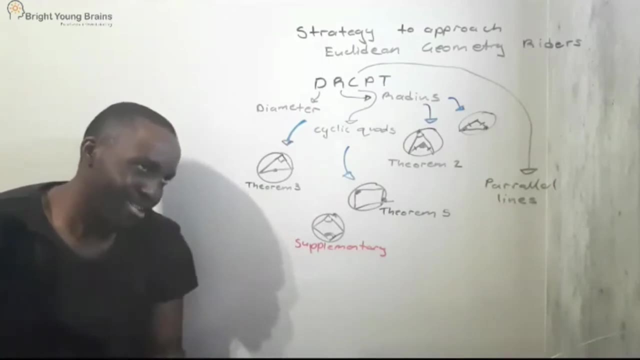 So that's what C does. P refers to parallel lines And I hope I spelled parallel correctly. I think parallel has one R. Yeah, that maybe looks better. So yeah, spelling an I Anyway. so P stands for parallel lines, And whenever we think of parallel lines, 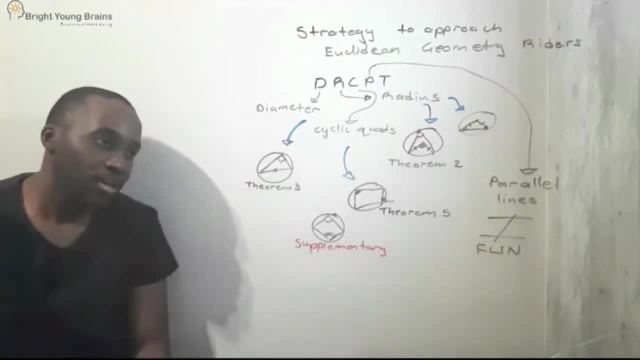 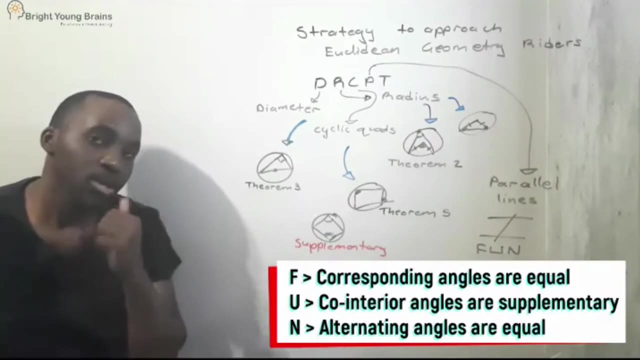 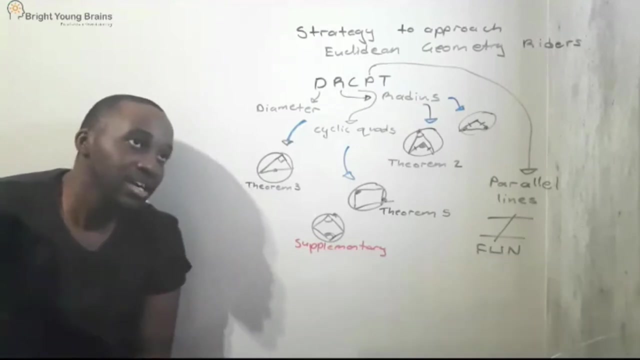 we will obviously need to remember fun: F for corresponding angles, U for co-interior angles and then N for alternating angles. So that's what the P will help you remember, or what you need to look out for T. you can almost guess it. T refers to tangents. So we know that with 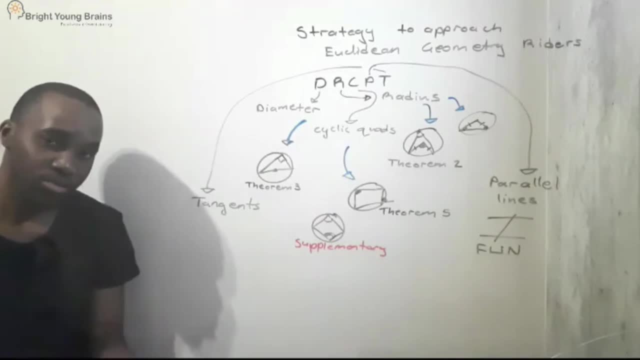 tangents. we have quite a few theorems, So one that you would be remembering is this theorem here. This theorem states that the radius of your circle will always meet a tangent at an angle of 90 degrees. Another tangent law is theorem 9,, the famous 10-code theorem, And then another tangent law. 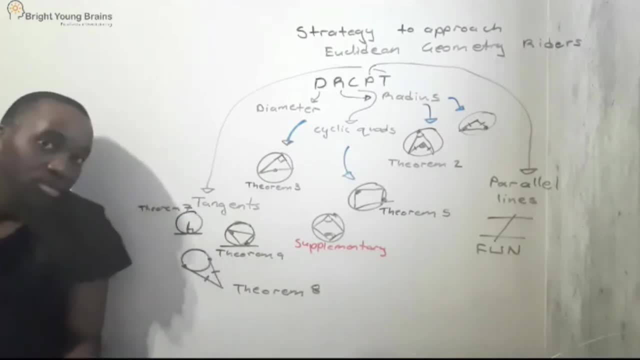 is theorem 8, which states that tangents from the same point are equal in length. So you can clearly see that Dr Cape Town is somewhat useful because it will help you keep in mind that D you need to think of diameters.